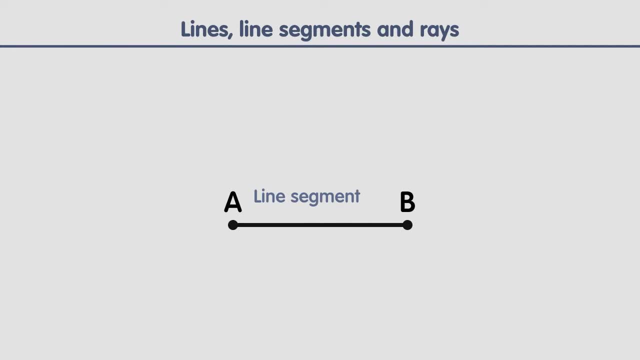 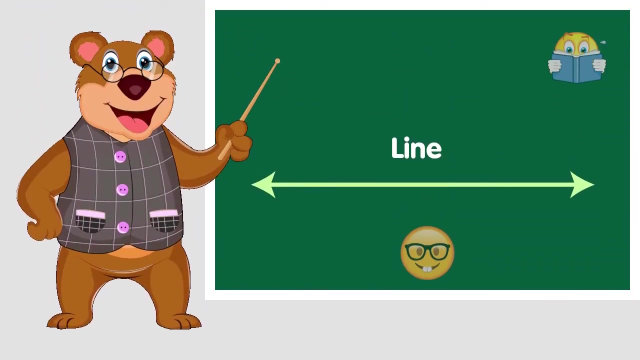 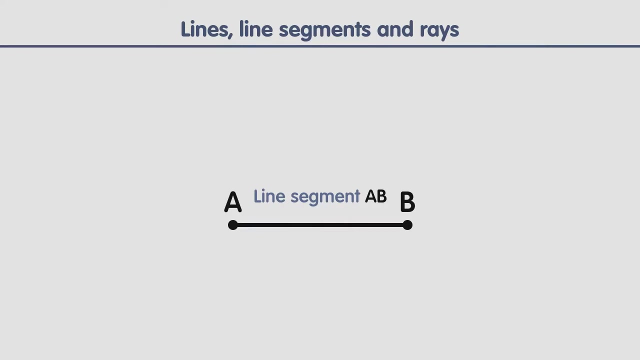 segment And we name it line segment AB. A line segment has a beginning and an end. It starts at one point and it ends at another. Now imagine that we draw another two points, Let's say point C and point D, And we join. 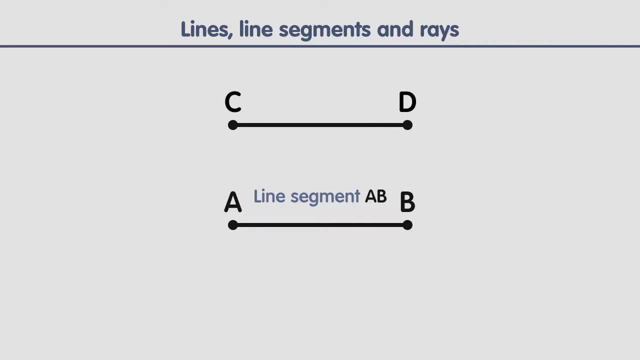 them, creating a line segment C-D. But now imagine that we extend this line segment forever in both directions. Well, this is not a line segment anymore. Instead we have a line. A line is a straight path that extends forever. Let's say point C and point D. So with these two points they are the same way. They will Fogen. Well, this is not a line segment. Instead we have a line. A line is a straight path that extends forever in both directions. to the point C. 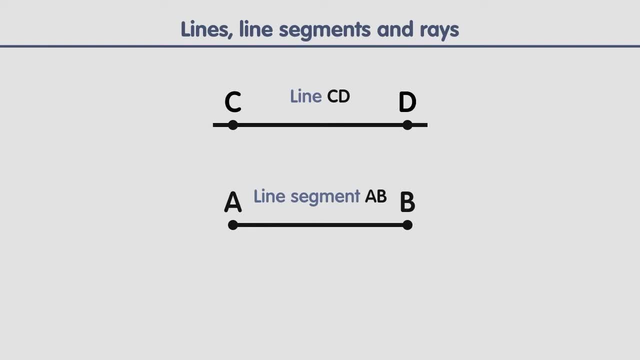 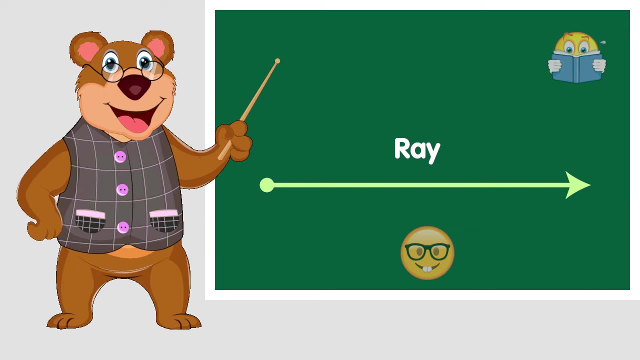 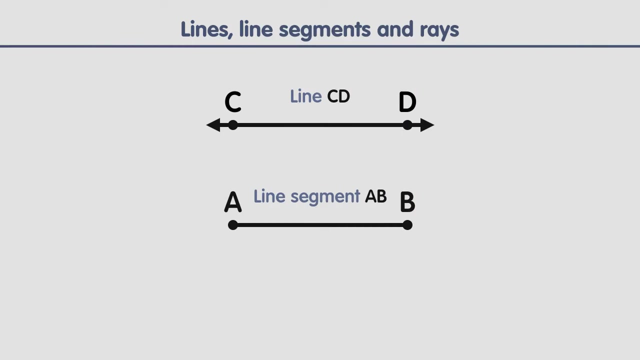 sections with no end points, But since we can't actually draw a line that goes on forever, what we do is draw an arrowhead on both ends of the line to show that keeps on going. There is one more special type of line that we need to talk about, and it's basically: 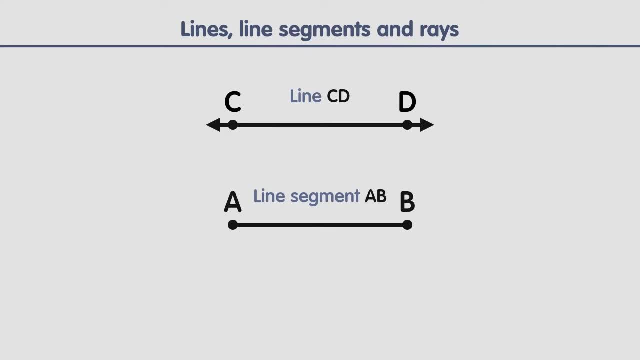 a combination of a line segment and a line. We call it a ray. To draw a ray, suppose we have a line segment with end points E and F. But now imagine that we extend this line segment forever in one direction, For example in the direction that goes from E to F And 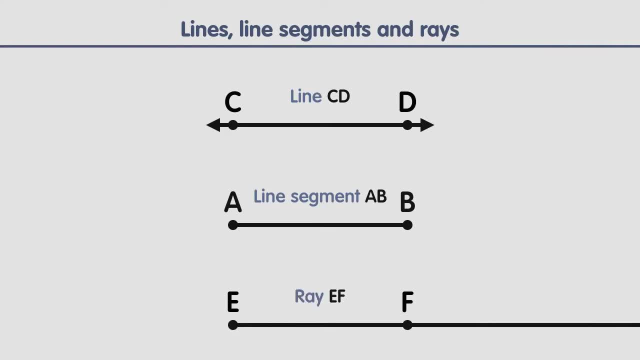 so we have created the ray EF. As we can see, rays have beginning points but no ending points. They just keep on going forever, But only in one direction, Similar to a line. we draw an arrowhead to indicate that the ray continues in that direction. 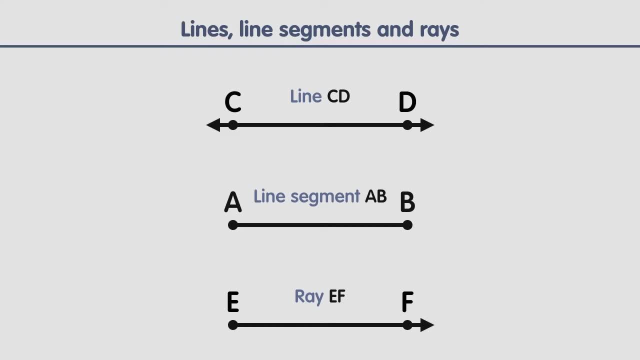 Each of these three types of lines has a shorthand way of writing it. Instead of writing line segment AB, we can just write AB with a line over the top. And instead of writing line CD, we can write CD with a double arrow line over them. And finally, instead of writing, 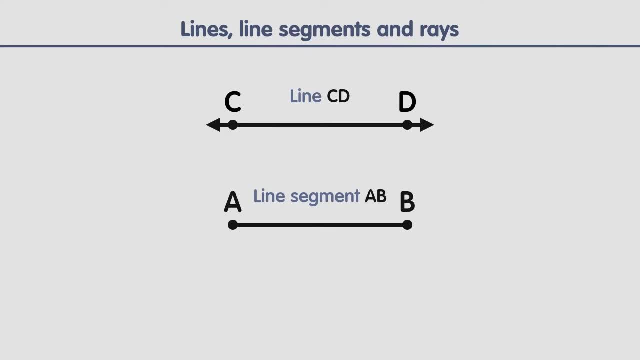 a combination of a line segment and a line. We call it a ray. To draw a ray, suppose we have a line segment with end points E and F. But now imagine that we extend this line segment forever in one direction, For example in the direction that goes from E to F And 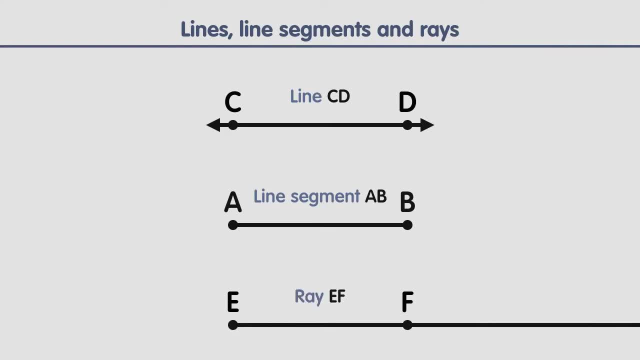 so we have created the ray EF. As we can see, rays have beginning points but no ending points. They just keep on going forever, But only in one direction, Similar to a line. we draw an arrowhead to indicate that the ray continues in that direction. 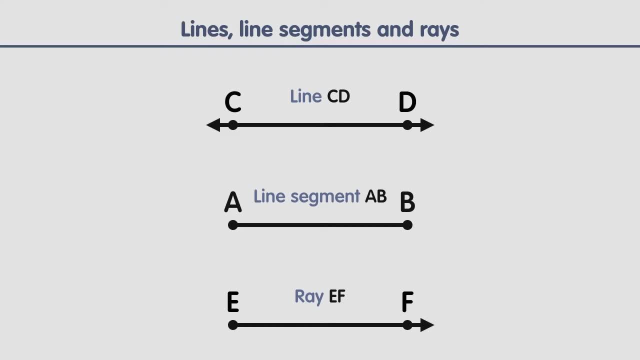 Each of these three types of lines has a shorthand way of writing it. Instead of writing line segment AB, we can just write AB with a line over the top. And instead of writing line CD, we can write CD with a double arrow line over them. And finally, instead of writing, 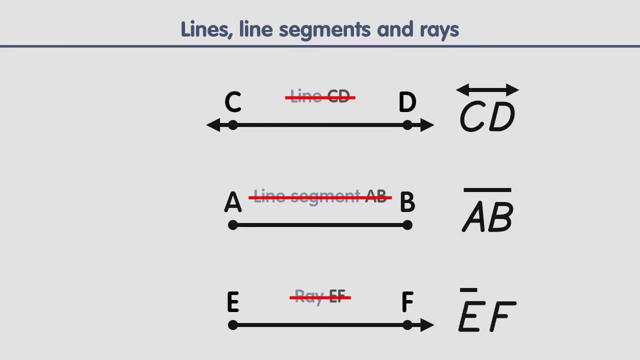 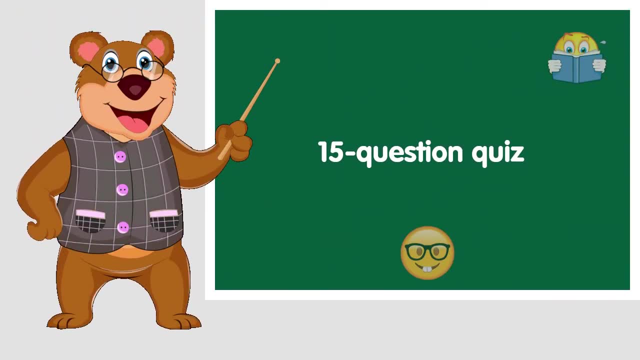 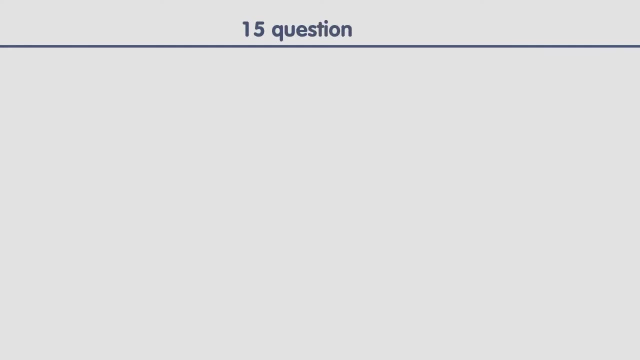 ray EF. we can just write line CD with a double arrow line over them. We can just write EF with a single arrow line over them. Which of the following diagrams is a line segment? That's right, The first diagram is a line segment as it has two endpoints without arrowheads. 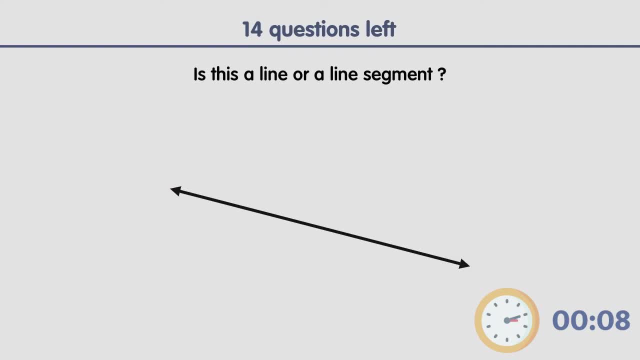 Is this a line or a line segment? Correct, It's a line, as it has an arrowhead at both ends. Which of the following options is the right way to denote the given field? The first one is a line segment. The second one is a line segment. The third one is a. 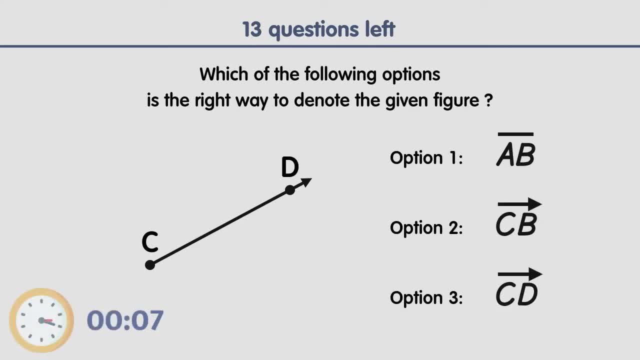 line segment. The fourth one is a line segment. The fifth one is a line segment. The sixth one is a line segment. The sixth one is a line segment. Who was the first person to get started on something using? memorize examples of numbers. 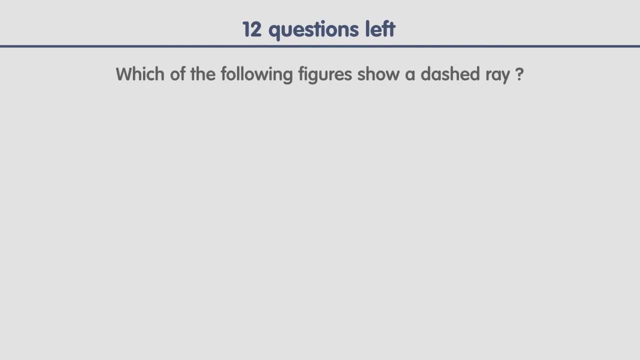 Finally, let's give a quick answer to that question. That's right. The answer is option 3.. Which of the following figures show a dash tray? Correct Figure B is showing a dash tray. correct Figure B is showing a dash tray. 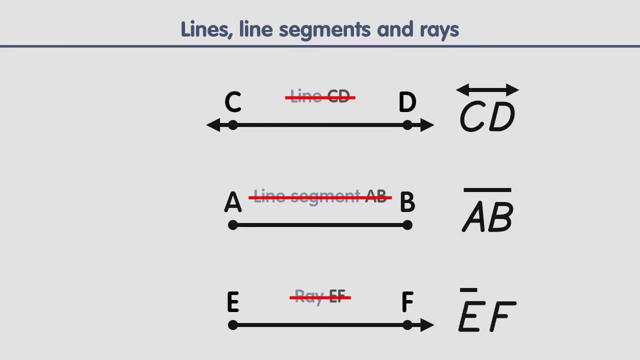 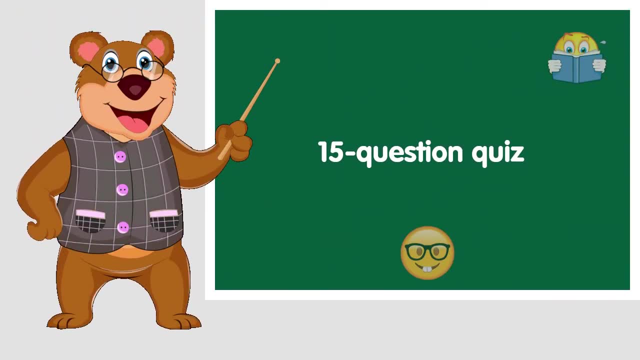 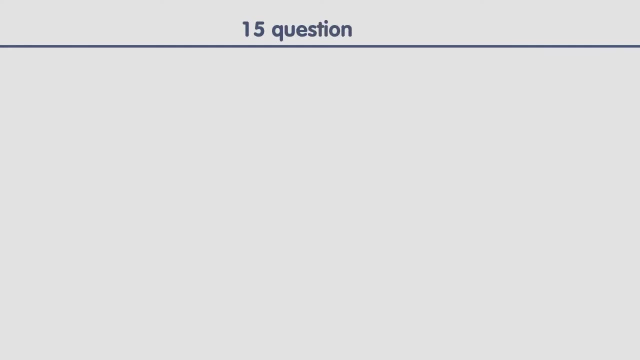 ray EF. we can just write line CD with a double arrow line over them. We can just write EF with a single arrow line over them. Which of the following diagrams is a line segment? That's right, The first diagram is a line segment as it has two endpoints without arrowheads. 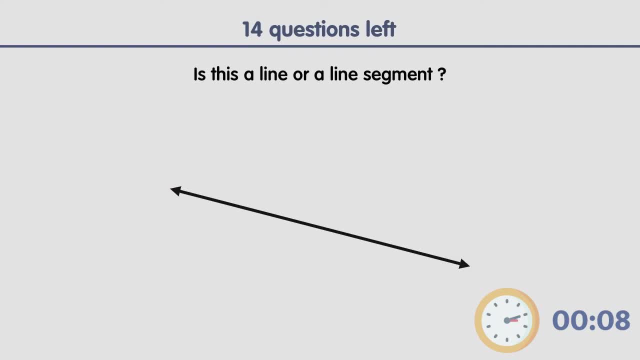 Is this a line or a line segment? Correct, It's a line, as it has an arrowhead at both ends. Which of the following options is the right way to denote the given field? The first one is a line segment. The second one is a line segment. The third one is a. 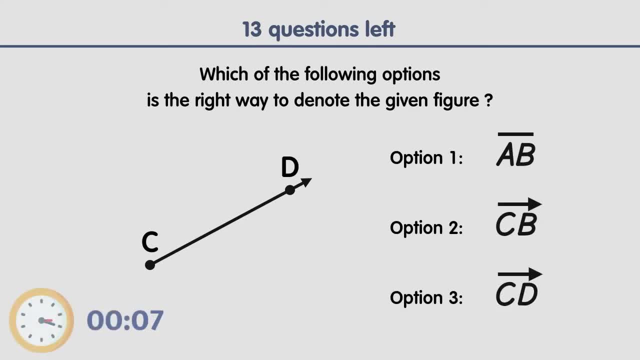 line segment. The fourth one is a line segment. The fifth one is a line segment. The sixth one is a line segment, If this is the right element. the third one is a line segment. The fourth one is a line segment. The fifth one is a ream segment. 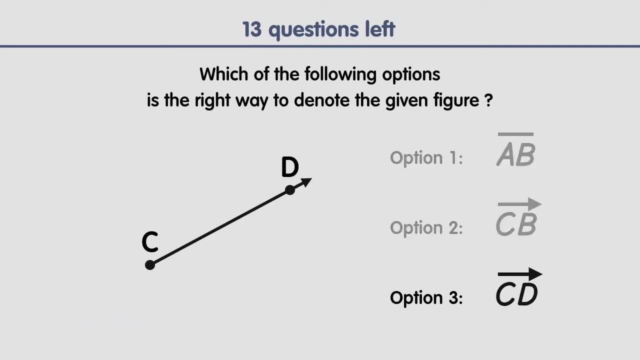 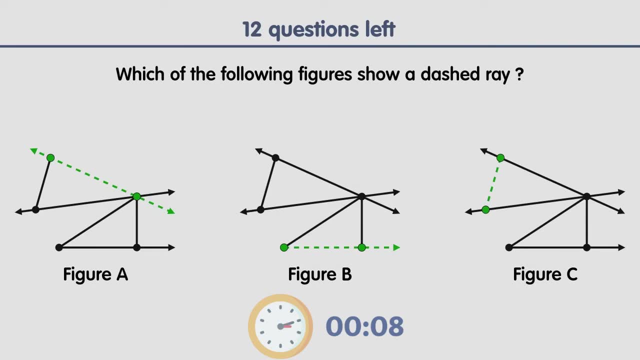 That's right. The answer is option three. Which of the following figures shows a dash tray? Correct. Figure B is showing a dash tray. Which of the following figures shows a disks؟? 生活- Correct. Figure B is showing a diskutray. 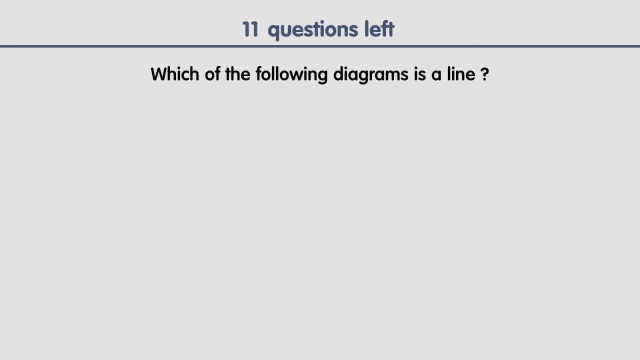 Which one of these figures shows the Divine lightning sontronies. This, Which of the following diagrams is a line? That's right. The first diagram is a line, as it has no endpoints and has an arrowhead at both ends. Is this a line, segment or array? 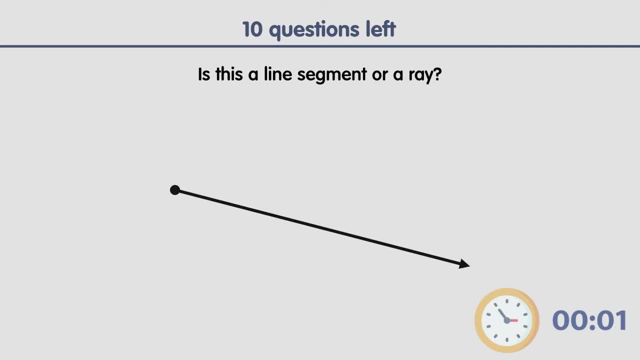 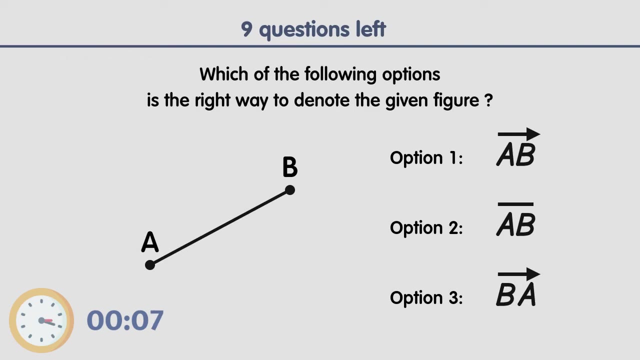 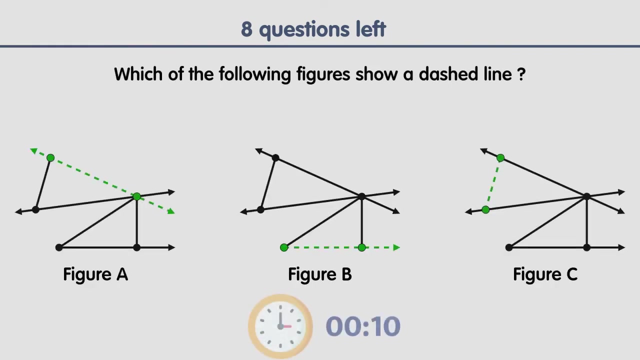 Correct Its array as it has only one endpoint and an arrowhead at the end. Which of the following options is the right way to denote the given figure? That's right, The answer is option 2.. Which of the following figures show a dashed line? 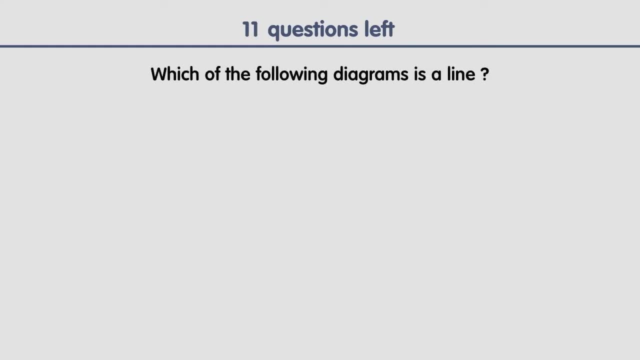 Correct. Figure B is showing a dash tray. Which of the following two figures have a dash tray? Which of the following diagrams is a line? That's right. The first diagram is a line, as it has no endpoints and has an arrowhead at both ends. 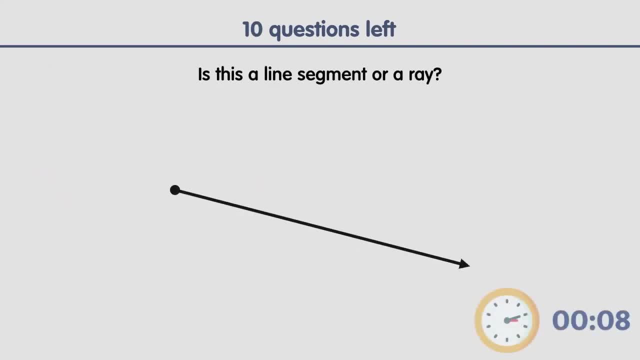 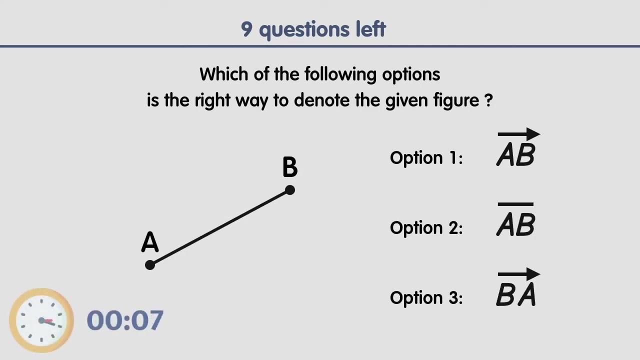 Is this a line, segment or array? Correct Its array, as it has only one endpoint and an arrowhead at the end. Which of the following options is the right way to denote the given figure? That's right. The answer is option 2.. 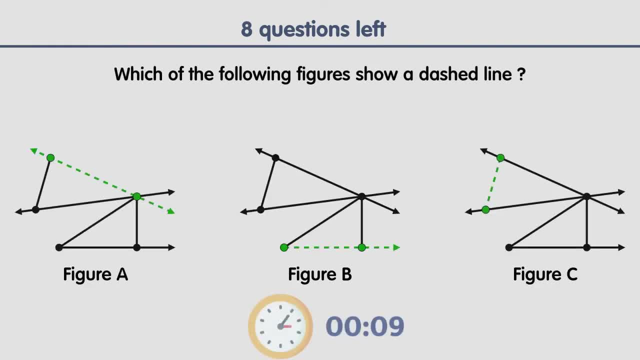 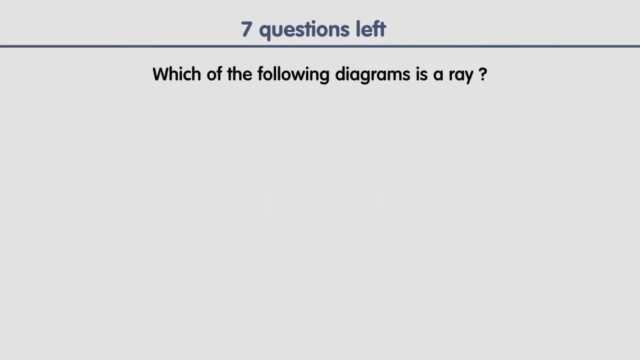 Which of the following figures show a dashed line? Correct: Figure A is showing a dashed line. Which of the following diagrams is array? That's right. The second diagram is array, as it has a start point and an arrowhead to show that it continues. 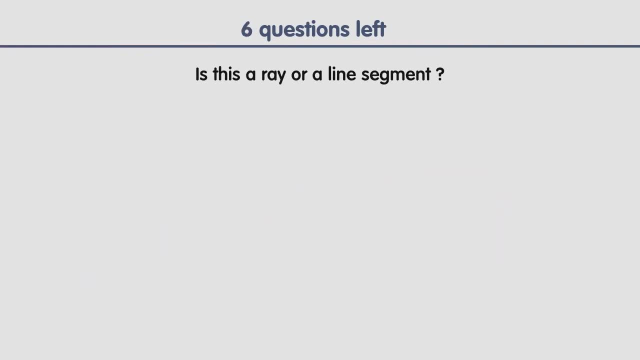 in that direction. Is this array or a line segment? Correct, Its a line segment, Since it has two endpoints without arrowheads. Which of the following options is the right way to denote the given figure? That's right. The answer is option 1.. 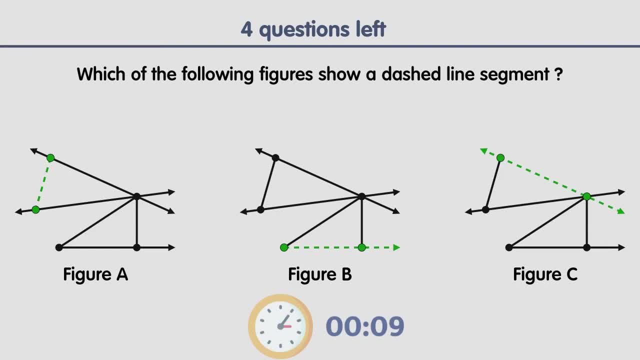 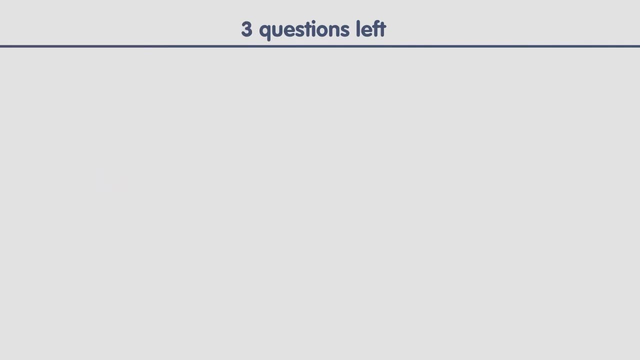 Which of the following figures show a dashed line segment? Correct Figure A is showing a dashed line segment. Which of the following options is the right way to denote the given figure? That's right. The answer is option 2.. Which of the following figures show a dashed line segment?